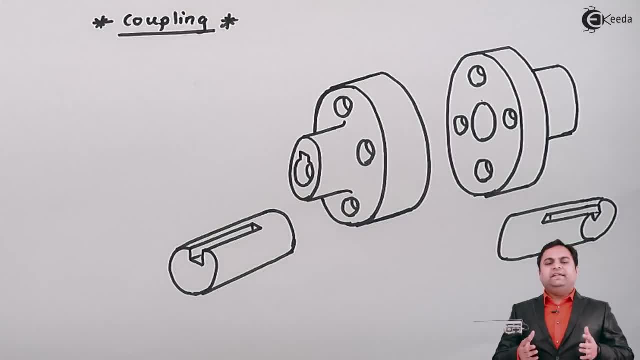 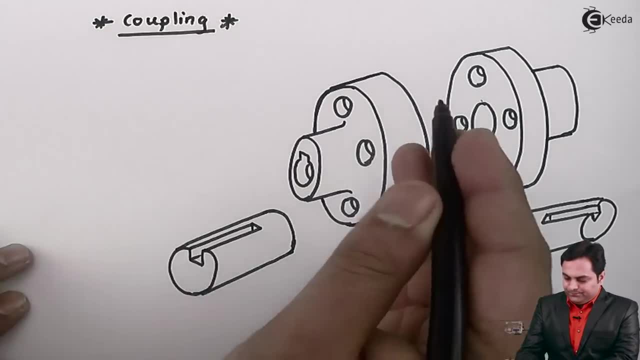 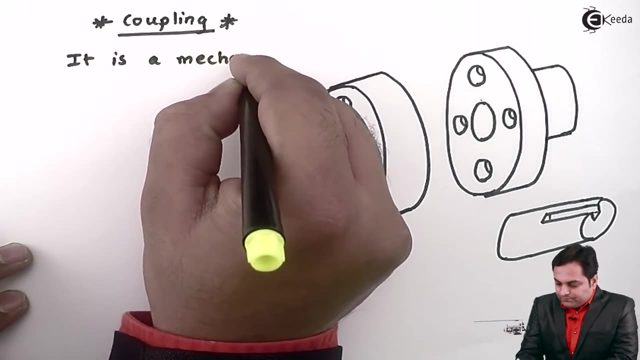 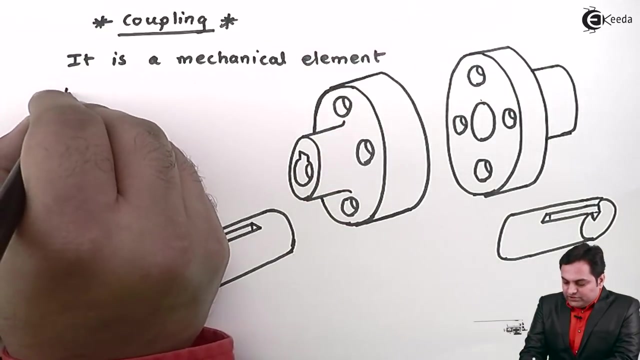 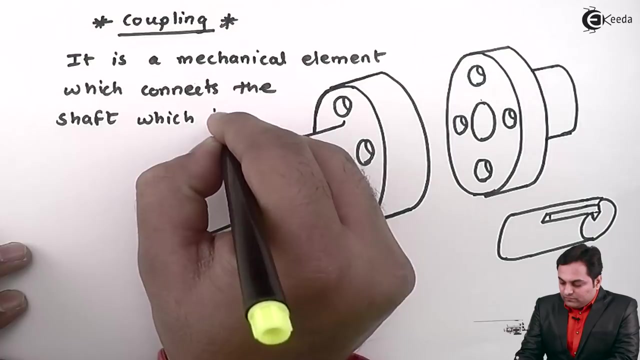 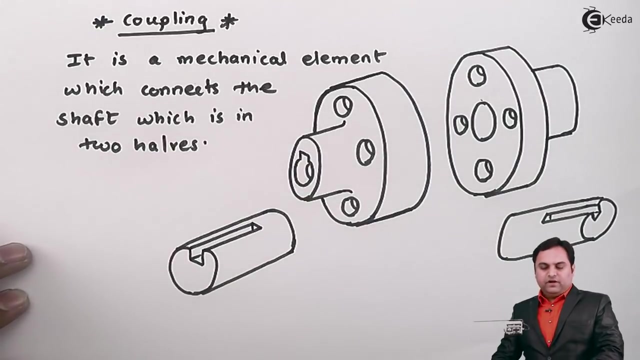 we just divide it into two halves and then connect those two halves by using the device called as coupling. So I will say that coupling it is a mechanical element which connects the shaft which is in two halves. So here I have written the definition of 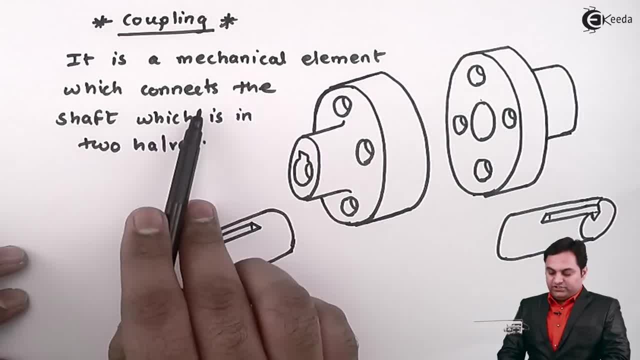 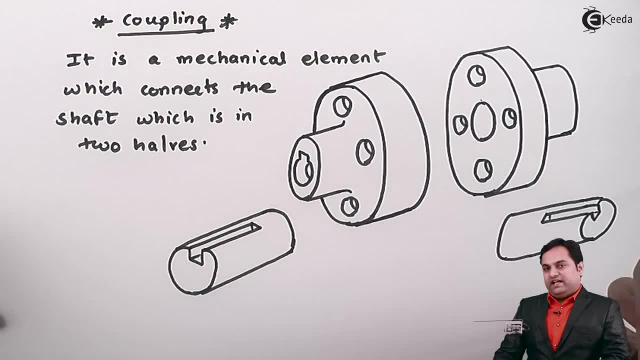 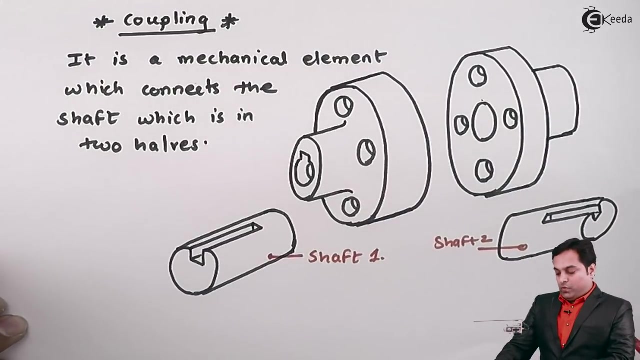 coupling, that it is a mechanical element which connects the shaft which is in two halves. Now how this connection takes place: Here I have a diagram in which there are two shafts, shafts- This I can say that it is shaft one, and here we have the second shaft. Now, when you want, 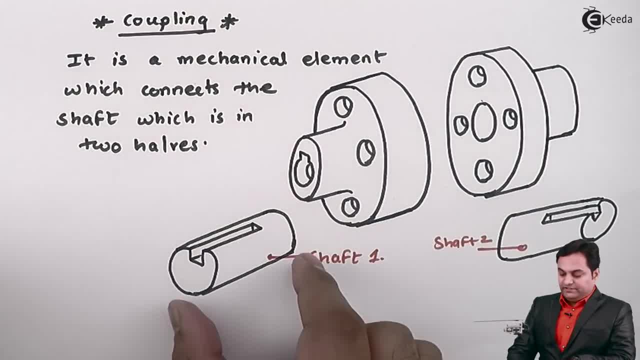 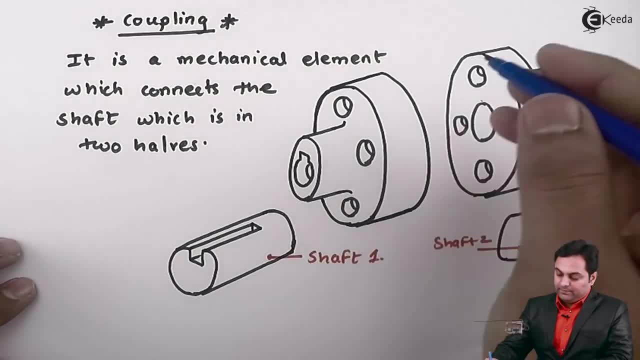 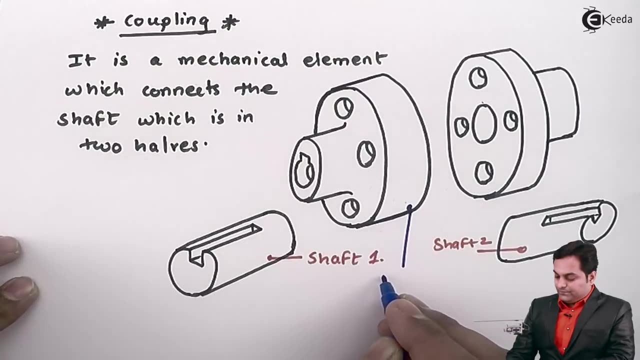 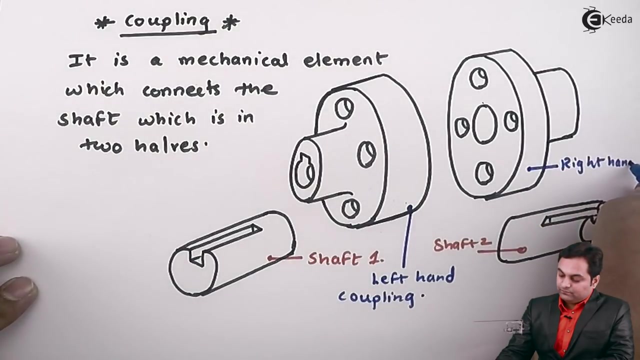 to connect these two shafts. in that case, we would be taking shaft one and inserting it into this device, which is nothing but called as the coupling, and here, since it is in the left hand side, I'll say that this is left hand coupling and here we have right hand coupling. Now how the connection takes. 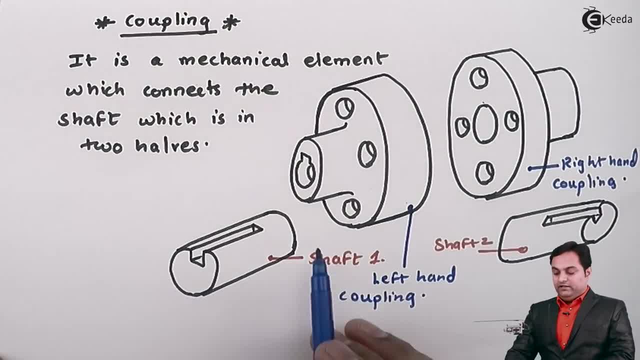 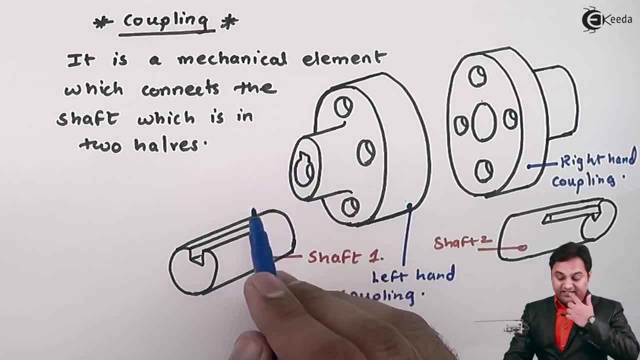 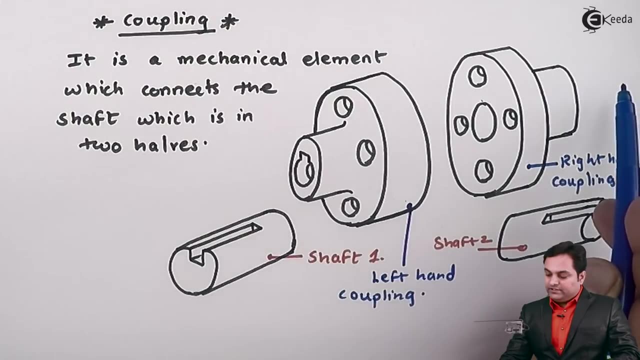 place We would be inserting shaft number one in left hand coupling, connecting it with a keyway. or here we have keyway, so we would be inserting the key which would go into the shaft and this hub. Next we will take shaft number two and connect it in the right hand coupling by using a key. 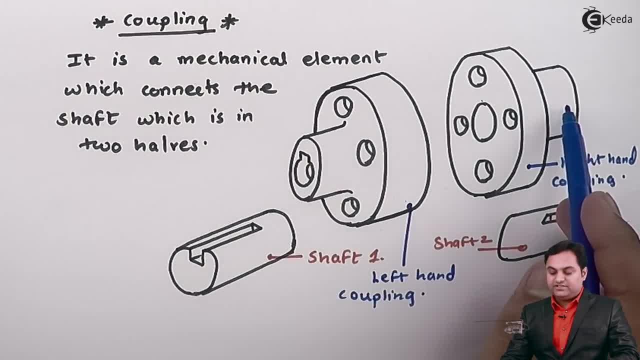 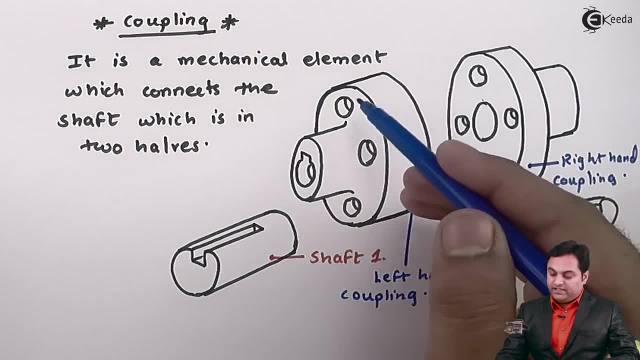 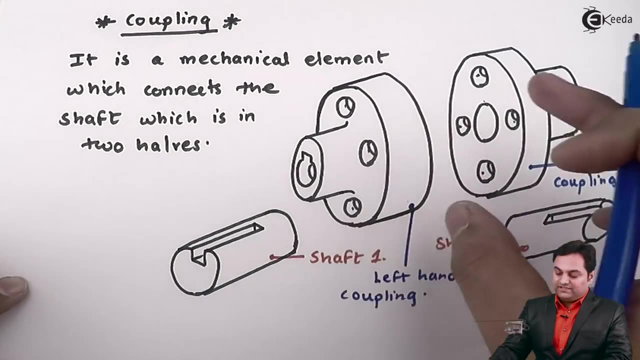 whose half portion is there in the shaft and half is there in this hub. When the shaft have been connected, we would be joining these two couplings and here, as we see, there are number of holes provided on the circumference of this coupling. So we would be matching or aligning these holes and 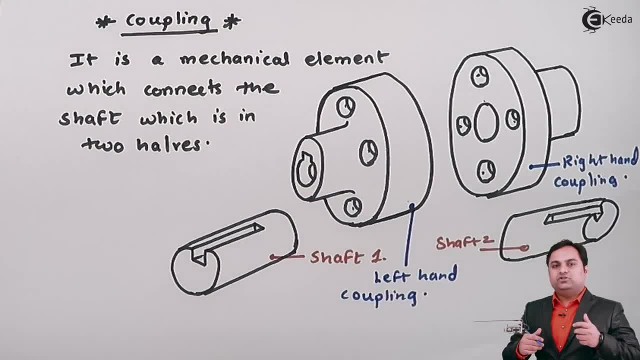 then we would be inserting bolts in that, bolts and nuts, so that the coupling becomes tight. It becomes a single connection. Now, if we give power to any one of the shaft, it would rotate the other shaft and the motion would be transmitted through this coupling. 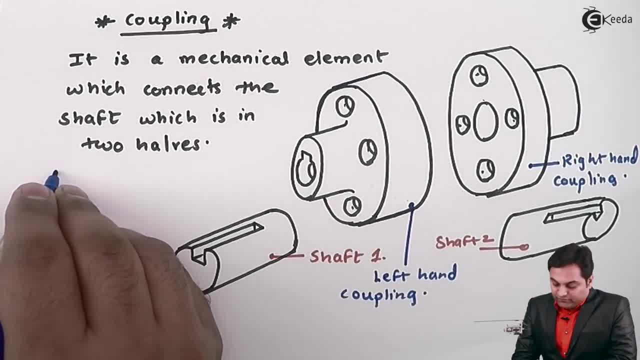 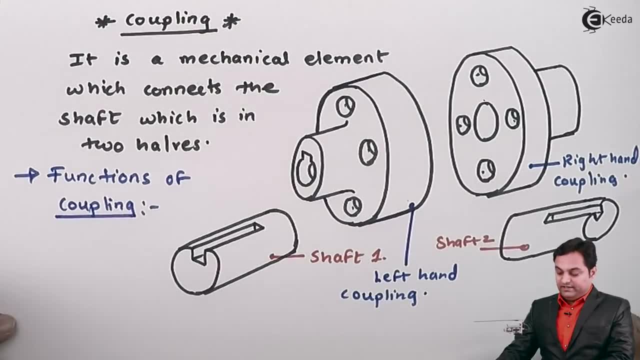 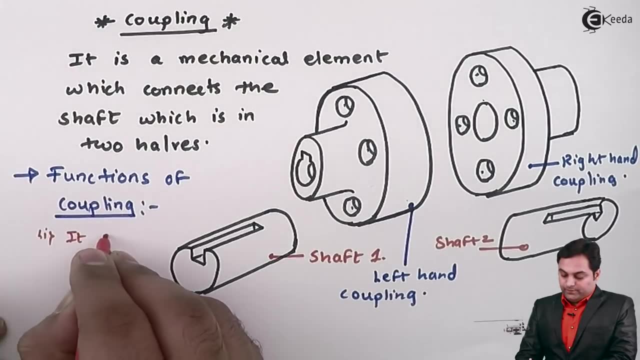 I'll say that functions of coupling. Now, when I'm defining the functions, I'll write down the first one: It should connect or align two shafts. That is the first primary function of a coupling or two shafts coupling. that it should connect or it should align, make in line two shafts. the 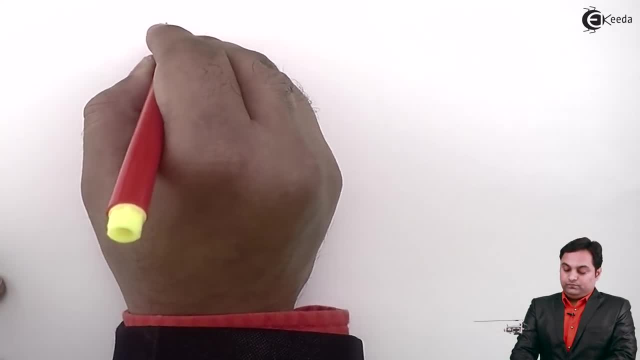 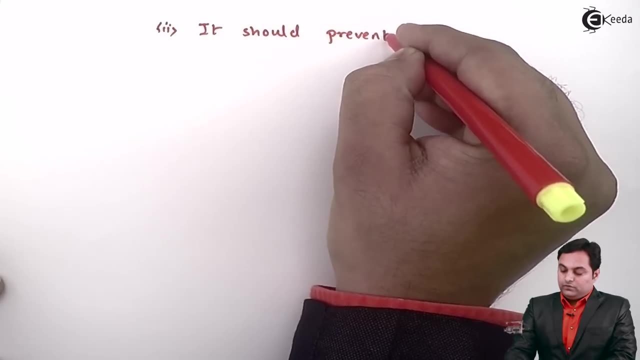 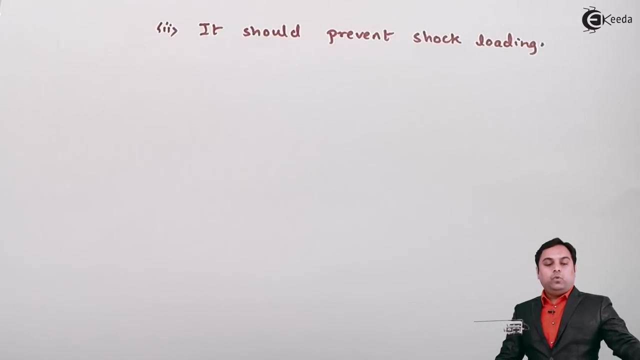 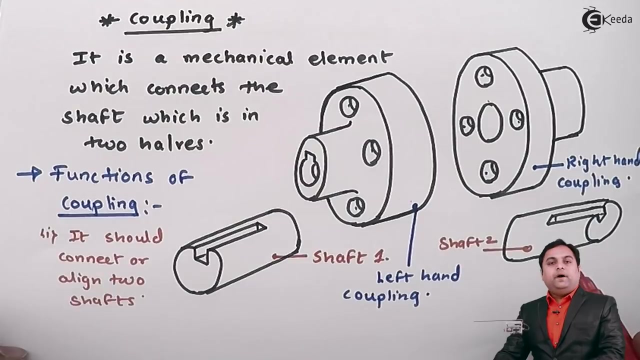 next point: it should prevent shock loading. see, the meaning of shock loading is that we will be giving power to any one of the shaft and when the power is transmitted to the other shaft, there is some amount of time gap. so it should not happen that suddenly the shaft starts rotating. it should attain the speed. 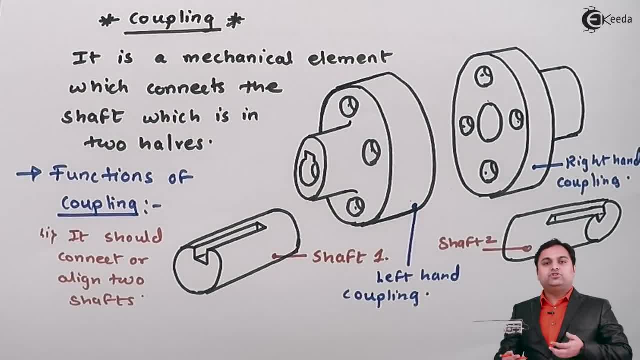 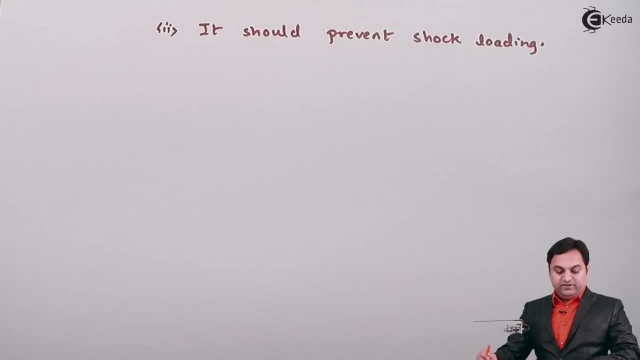 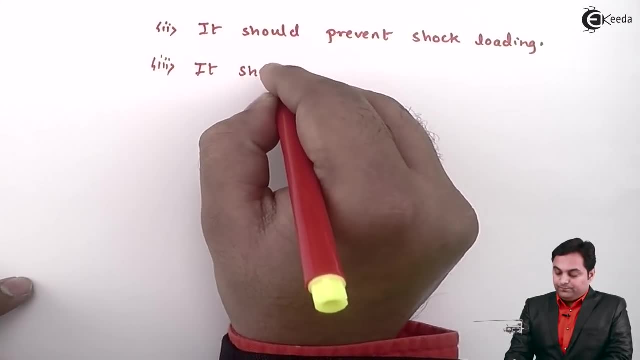 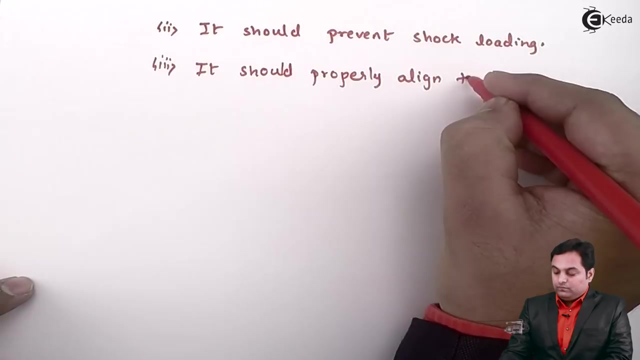 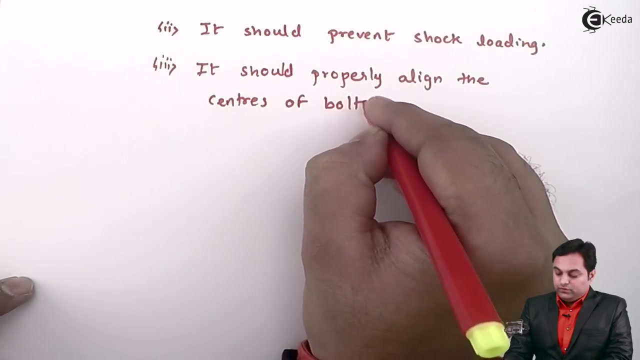 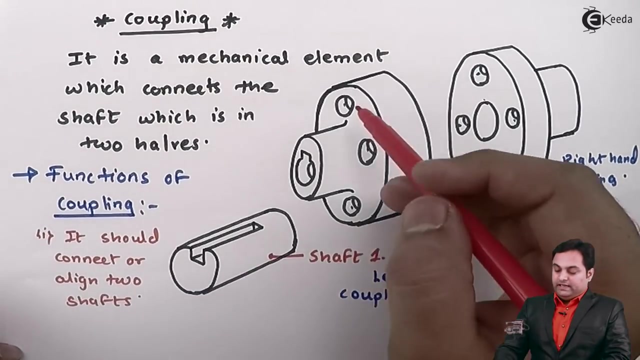 gradually. that is, if it starts with shock load, there are chances of shearing, breaking of the shaft, so it should prevent shock loading. so it should prevent shock loading. so it should prevent shock loading. next, it should properly align the centers of bolts. next, as we see, when you want to connect left-hand and right-hand coupling, in that case the 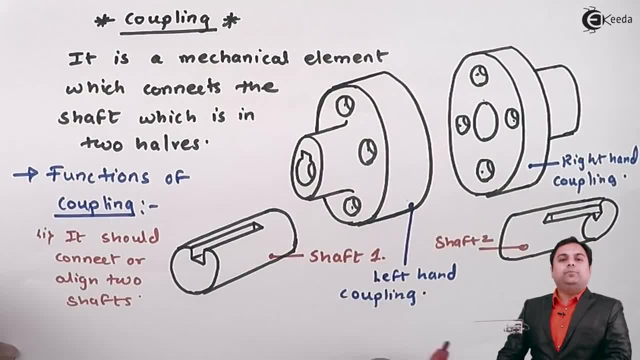 holes which are provided for the bolts. they should be properly aligned. then only the coupling would transferring power in a more simplified or more smooth manner. because if the centers are not matching then there are chances of the bolts to shear, to break, because one coupling- it would be rotating and the other one would.